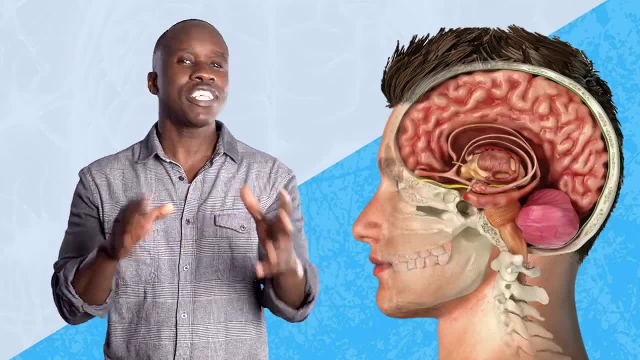 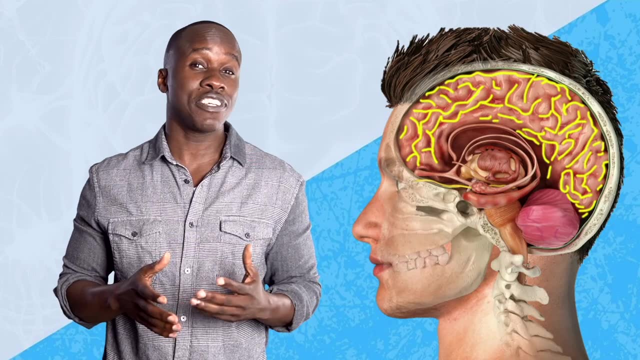 Well, your cerebrum is involved with that too. Now, the feature that you notice most about the surface of the brain is that it's wrinkled. Well, that entire wrinkled surface is called the cerebral cortex. That's the superficial part. 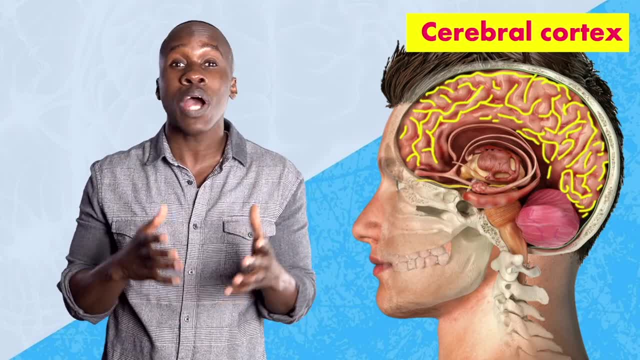 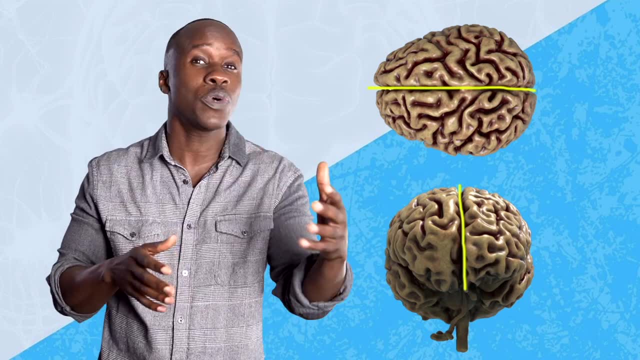 And you'll also notice that the cerebrum is divided into two halves. That separation part, this long line from the front all the way to the back that separates the cerebrum into the two halves, is called the longitudinal Longitudinal fissure. 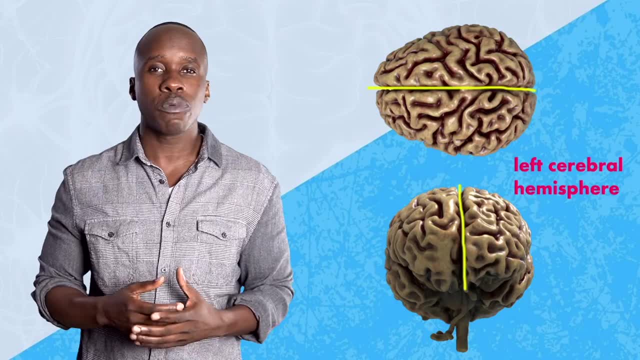 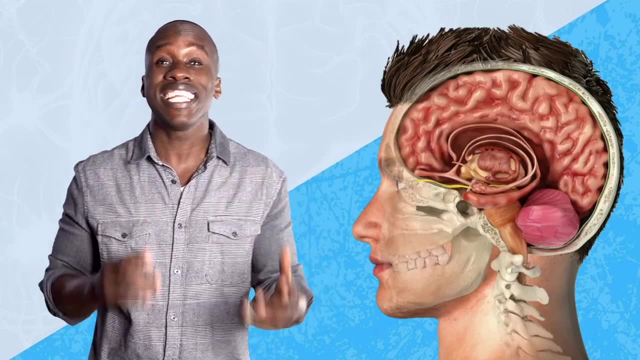 And the two halves are called hemispheres. You have the left cerebral hemisphere and the right cerebral hemisphere, commonly called the left and right brain. Now, those two hemispheres are actually connected by a bundle of nerve fibers that we call the corpus callosum. 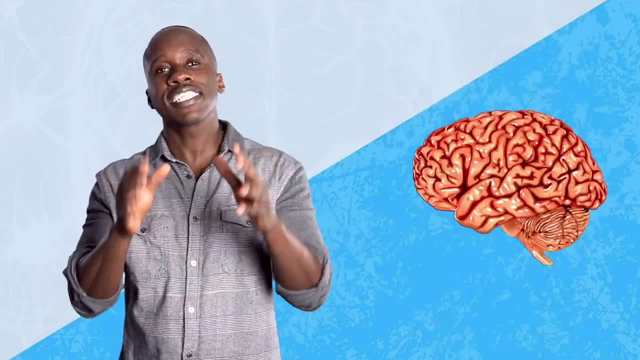 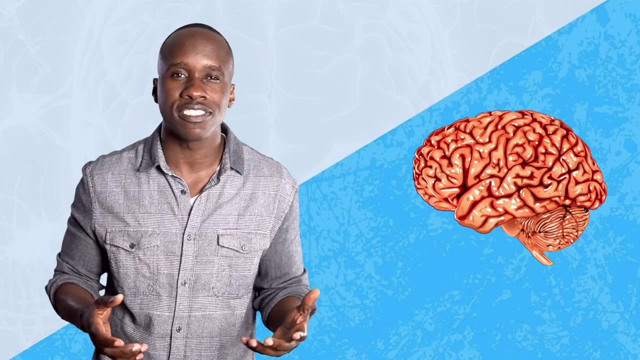 And this allows for the left and right hemispheres to communicate. Okay, let's get back to the cerebral cortex. As I mentioned, it's very wrinkled. It has a bunch of grooves and a bunch of ridges. The grooves are called sulci, which is the pleural 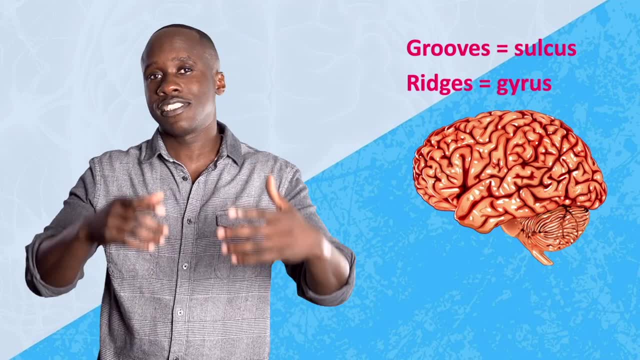 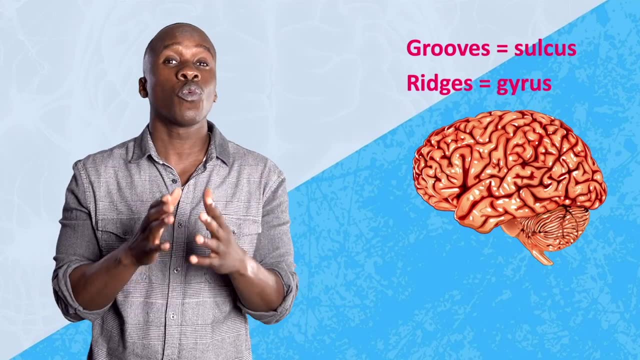 of sulcus and the ridges are called gyri, which is the plural of gyrus. This wrinkled structure, which basically involves the folding of the cortex, accomplishes one very important thing: It increases the surface area of the cortex of the brain. 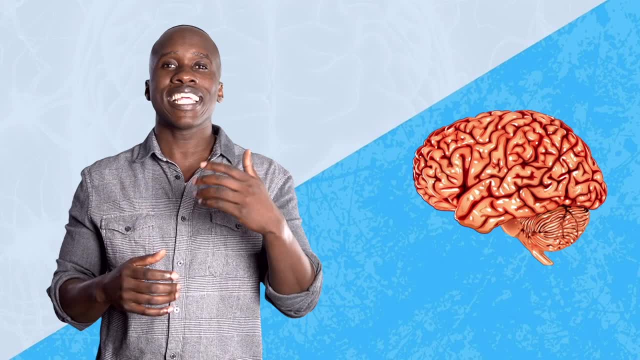 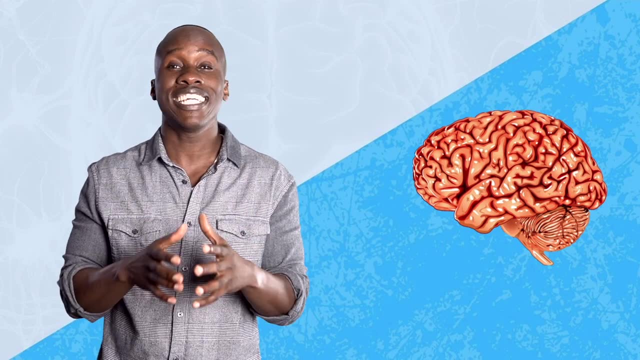 Now, as we look further at the cerebral cortex, we're gonna see that, in addition to all these smaller sulci, we also have two more distinct sulci that separate the cortex into distinct lobes. We have the central sulcus that separates the parietal lobe from the frontal lobe. 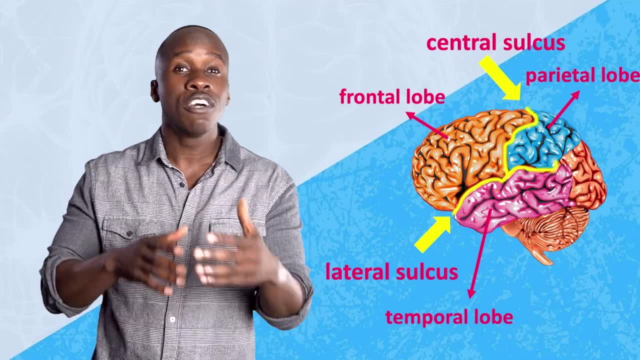 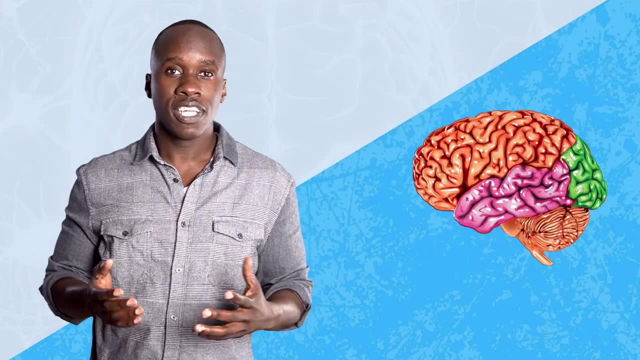 and we have the lateral sulcus which separates the temporal lobe from the other lobes. There's also one other lobe, that's the occipital lobe, That's the posterior region of the cortex. Now, looking at the brain from the outer surface, 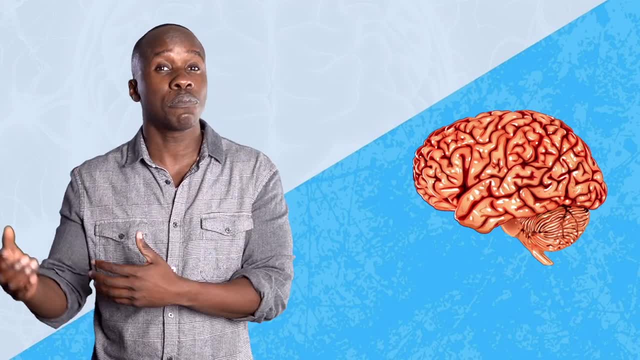 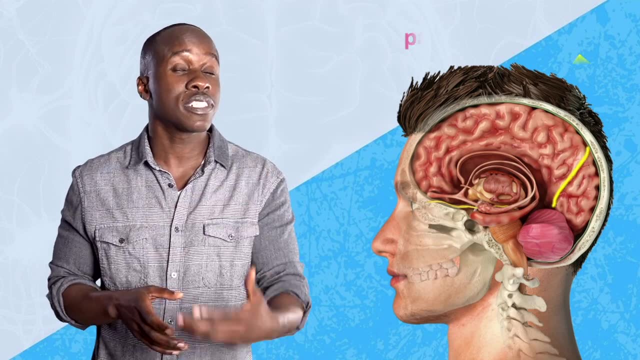 you don't see any major sulcus that's separating the occipital lobe and the parietal lobe. But if you were to look from the medial surface you'll see that there's a parieto-occipital sulcus. 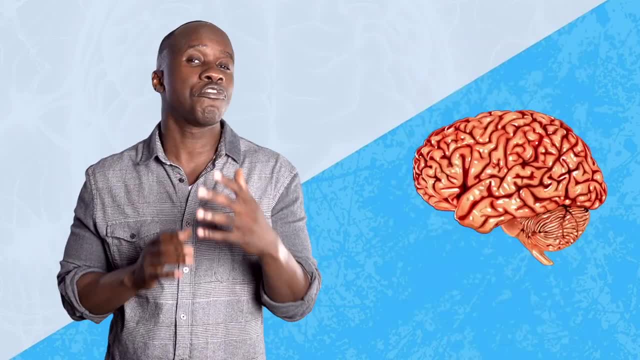 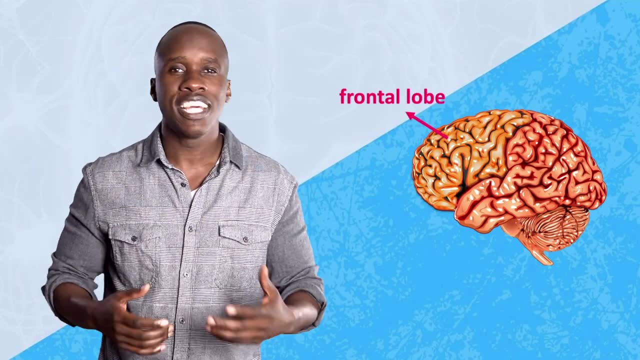 Okay, so those are the parts of the cerebrum, But what are their functions? Let's dig into that a little. The frontal lobe: this is the part that's involved with higher level processing, Things like thought, reasoning, planning things out.